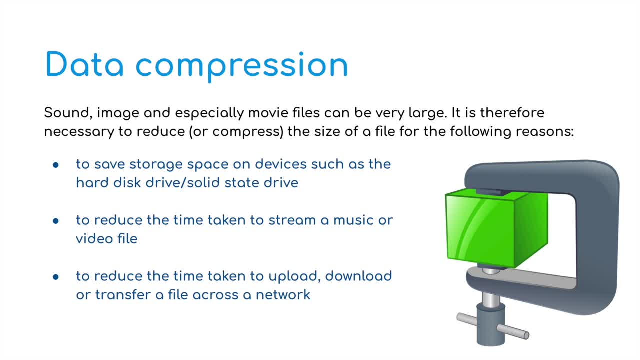 therefore necessary to reduce or compress the size of these files for any of the following reasons. We might need to save storage space on our devices If we're using a MacBook or a laptop, for example, which contains a hard disk or a solid-state drive, it's 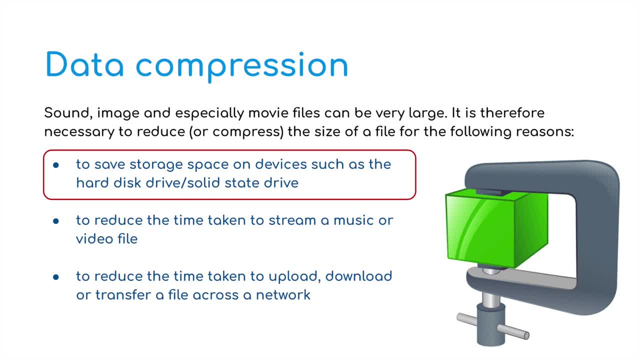 only a specific size, maybe one terabyte or maybe even less. So the more we put onto that, the quicker it's going to fill up. So if we reduce the size of these files, then obviously we can fit more on it. Secondly, we might need to reduce 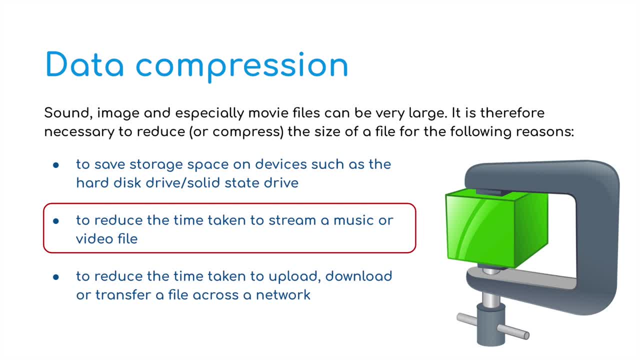 time taken to stream a music or a video file. If we've got a very reliable large file that we're trying to watch on our mobile phones or our portable devices, it might suffer in terms of the internet connection. It might do something called buffering, where it keeps having to stop and start download. 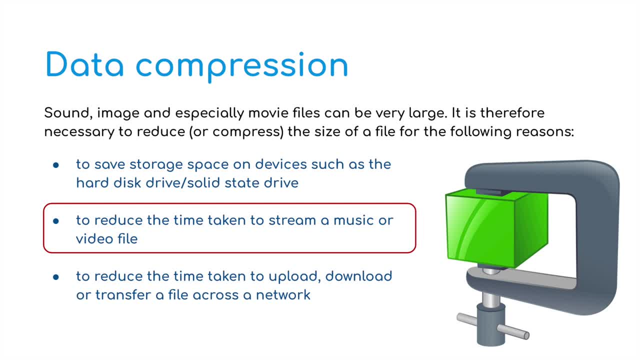 the information from the music or video file and it might be pausing and stopping and causing all sorts of problems, which is obviously going to lead to spoiling our enjoyment. Thirdly, we also need to reduce the time taken to upload, download or transfer a. 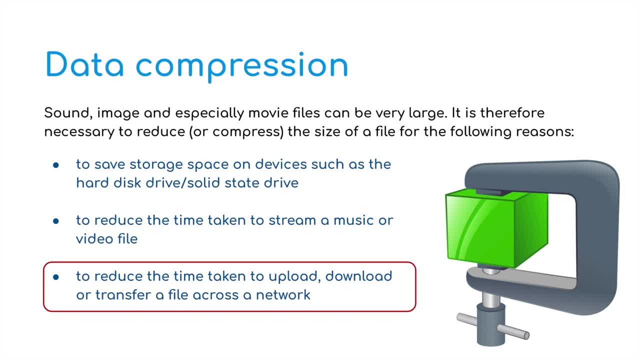 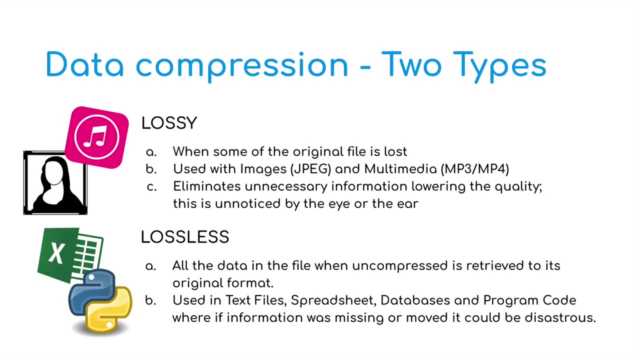 file over the internet. If you've got a very large file, it's obviously going to take a longer time to get that file to where it needs to be or to download it onto your computer. There are two main types of data: compression and the clues in the name. 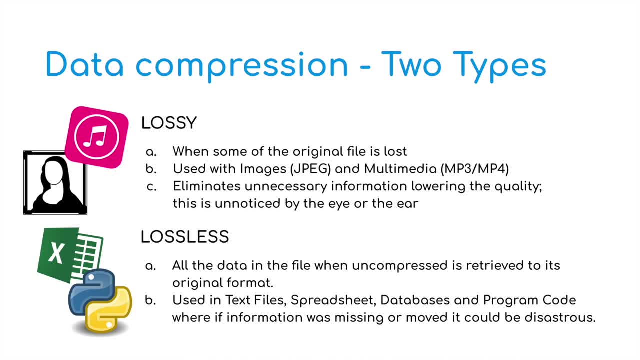 as to what exactly they do. The first one we're going to look at is lossy, and then, secondly, we're going to look at lossless. I'm just going to quickly go through an overview of each one, and then we're going to look at each one in a lot more detail. So lossy. 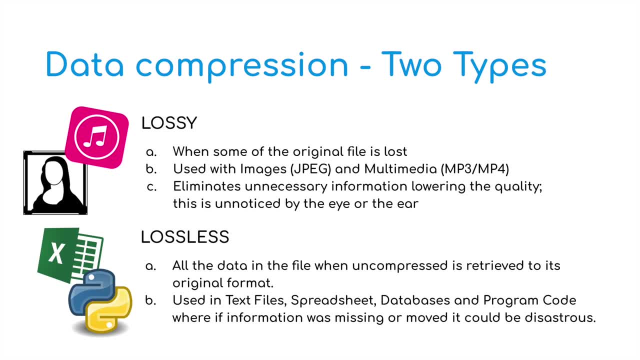 is when some of the original file has been taken away. it's been removed. This may affect the quality slightly. It's used with images such as jpegs and it's also used in mp3 and mp4 compression. It eliminates unnecessary information. so, yes, it lowers the. 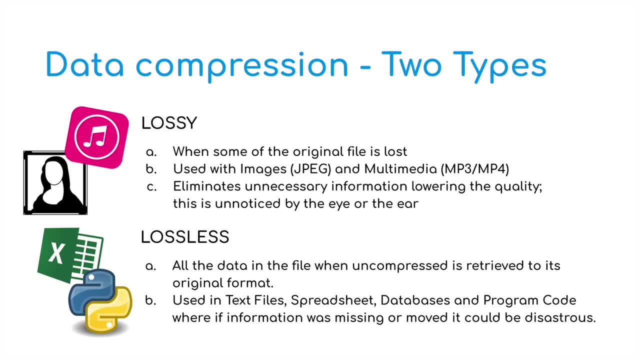 quality, but this generally goes unnoticed by our eyes or by our ears when we listen to or look at this data Lossless compression works in a different way. All the data in the file, when it's been compressed, is received in its original format. So, although it's been compressed, none of 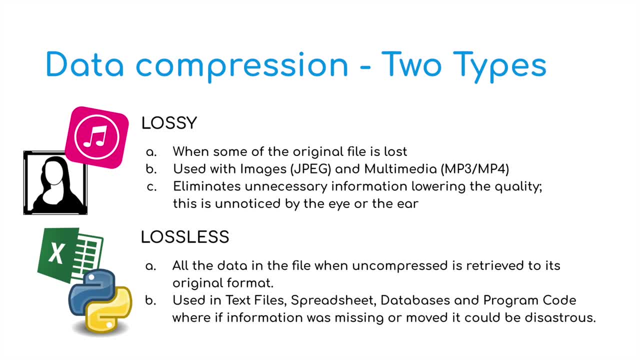 the original information has been removed. It's used for text files, spreadsheets, databases and program code where, if any information was missing or moved, it could be disastrous. I mean, you couldn't send a spreadsheet to a personal essay and it didn't have any results in it, or it had a missing column with important data or bits. 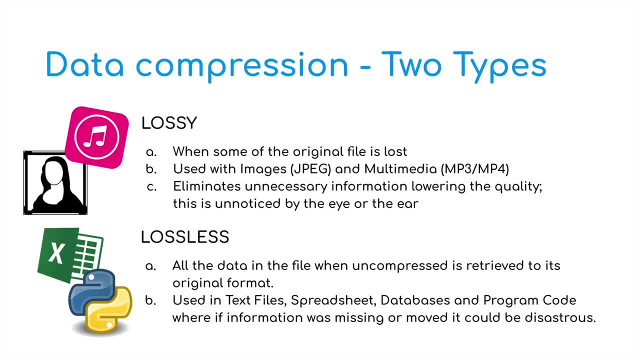 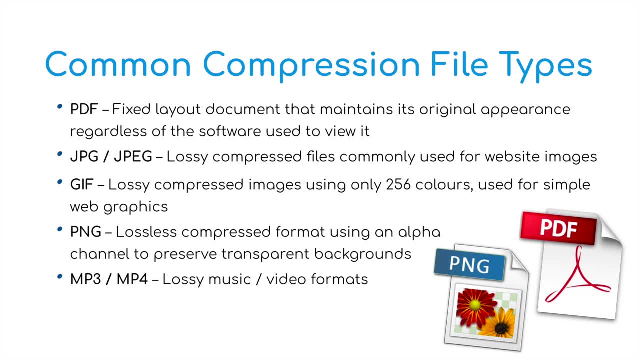 of data had been taken out, So that must arrive to the receiver intact, and that's when we'd need lossless compression. Here we have some file types, some compressed file types that I've put together You may be familiar with. we start with a pdf, a type of lossless compression used to transport. 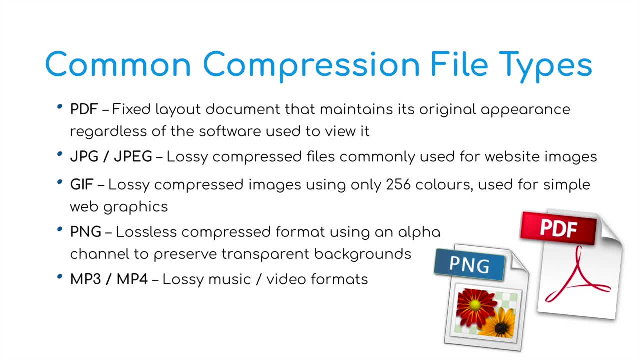 documents- transfer documents between different computers. There's no constraints in terms of what software you have on your computer. We've got the jpeg, which is an image file which is used generally for web pages, and this uses lossless compression. We've mentioned it before. 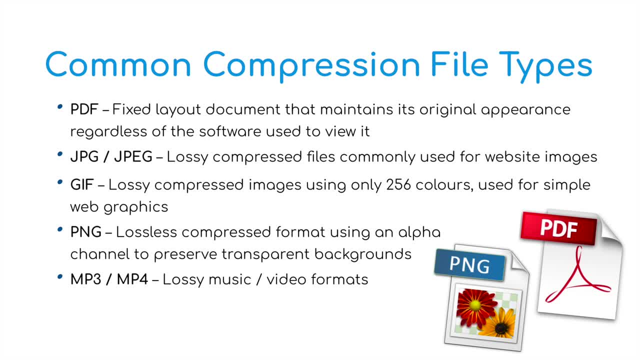 Similarly, we've got the gif, which uses again lossy compression but is restricted to 256 colours. You'll have seen this for memes and animated gifs. The png file, a popular file format on websites, is lossless compression, but it also has an alpha channel which preserves 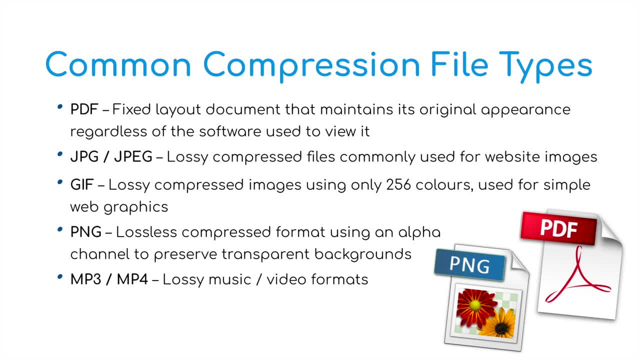 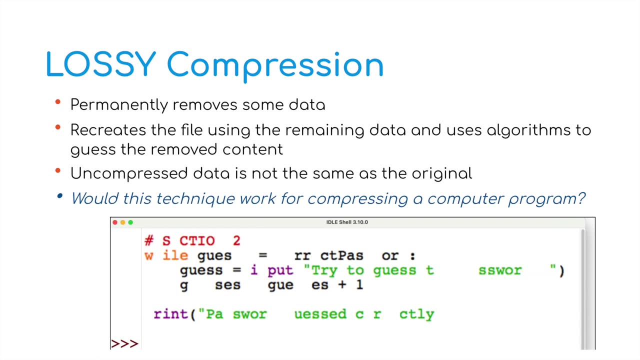 the transparent background. And then we have mp3s and mp4s, which both use lossy compression for music. So we'll talk in more detail first of all about lossy compression. This type of compression permanently removes some data. We don't get it back. If we compress a file, then we uncompress. 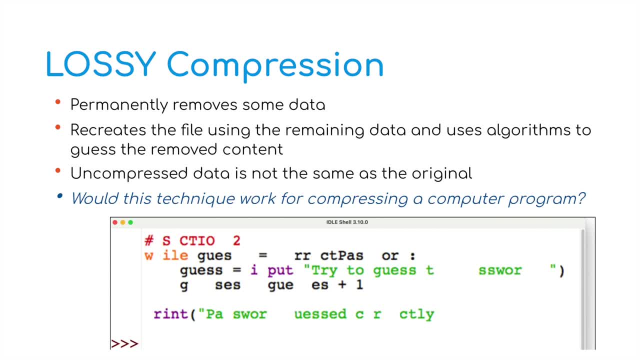 it data has been removed. It recreates a file using the remaining data and uses algorithms to guess the removed content. Uncompressed data is not the same as the original. I've got an example here of a python file I've created. Obviously, if we compress this, 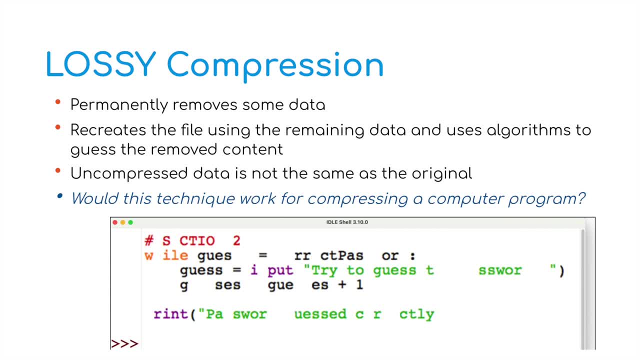 python file, we might lose some of the data. I've gone a little bit overboard, but you can see that lossy compression would not be used. It wouldn't be possible to use that. This program simply wouldn't run, and it would be a similar thing for a spreadsheet or database. 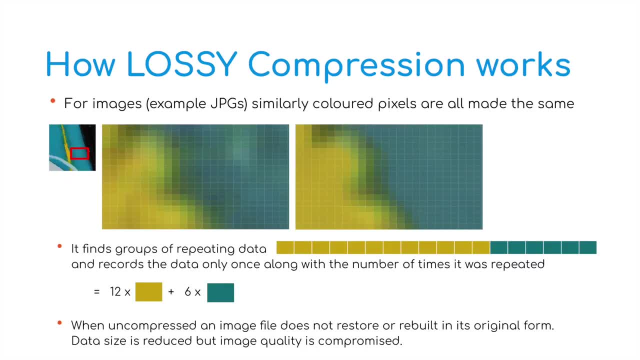 or something along those lines, Even a book. Here this jpeg. if we zoom right in to the coloured pixels, what it's doing is grouping similar pixels together or merging them into similar colours. it's reducing the colour depth. It also finds groups of repeating data. 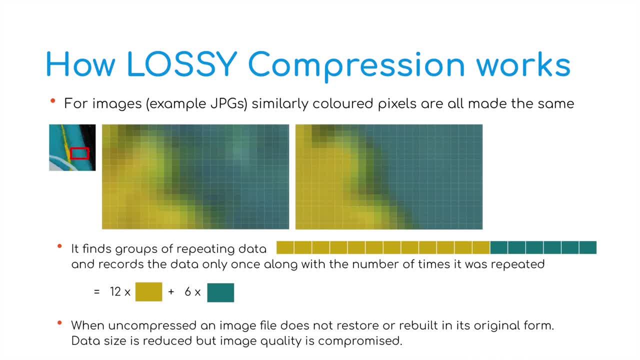 in this case this orangey, yellow and green. It only records data only once along the number of times we've seen that particular colour. So, for example, this particular line has 12 golden and would have 6 green If we use bomf to look up a approximate number of Holocaust sacrifices and gets a death rate. 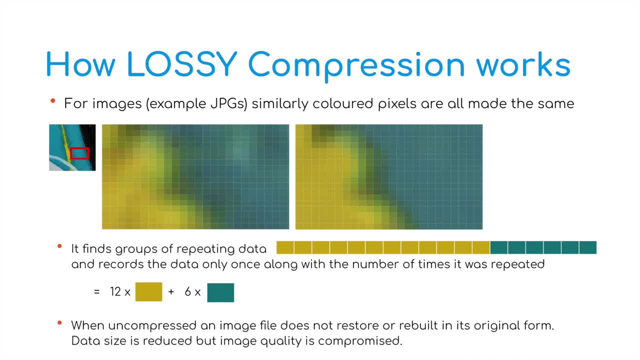 out of our data, we'll have a number of deaths. We just don't get a lot of deaths and therefore screen, When uncompressed, an image does not restore- as we mentioned before- or rebuild to its original form and the data size is reduced, but image quality can also be compromised. 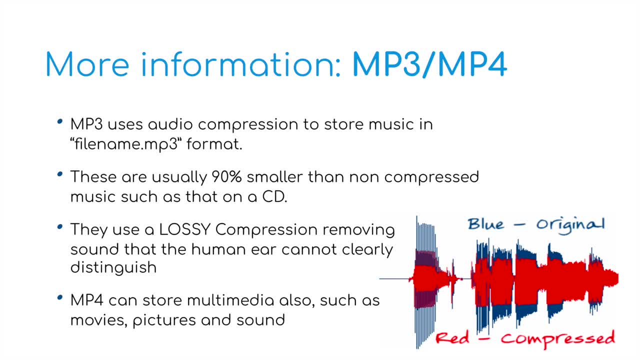 In terms of MP3s and MP4s. an MP3 audio compressed file, a music file, is stored as an MP3, so you'll be familiar with these, and they can reduce a music file right down to almost 90%. 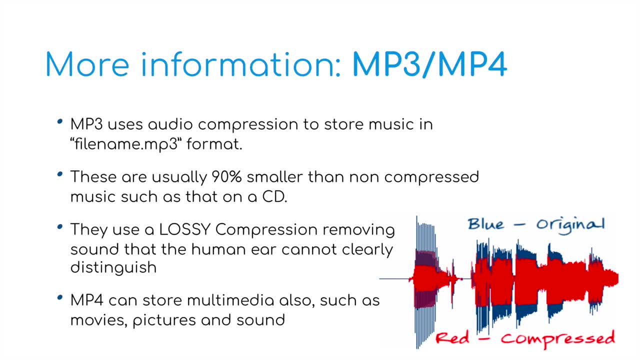 smaller than its original format when you might find on a CD something like a FLAC file. They use a lot of compression and they remove the sound that we can't hear. So if you look at the little diagram, we've got all the blue in the original file is gone Something if 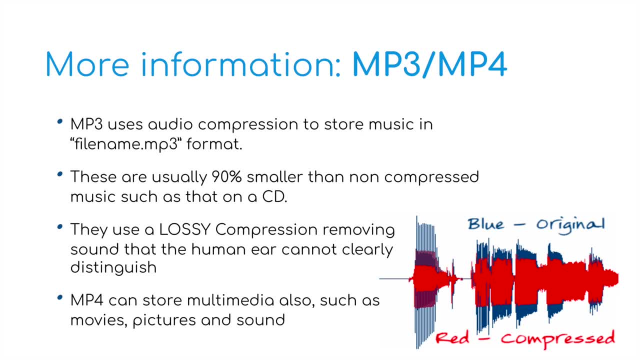 we say something like A dog whistle. We cannot hear it, but obviously we can whistle and the dog comes back. It's a sound that we can't distinguish and therefore it wouldn't be needed. MP4 obviously works. 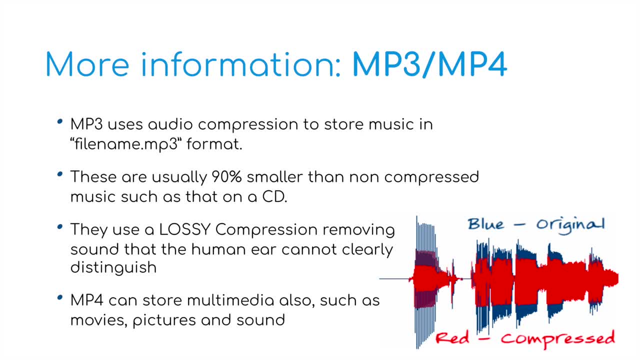 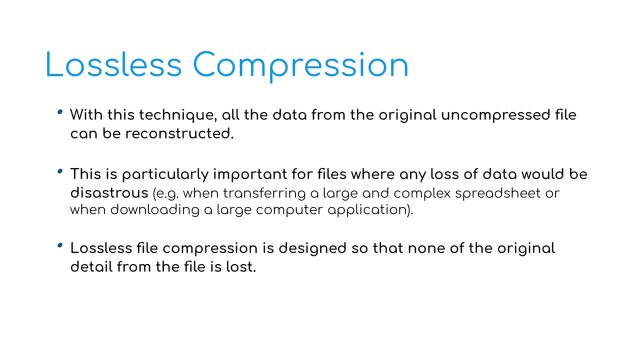 in a similar way in terms of what it's removing to reduce that file down. Move on to lossless compression. Okay, so what is this? Well, with this technique, all the data from the original uncompressed file can be reconstructed. What you? 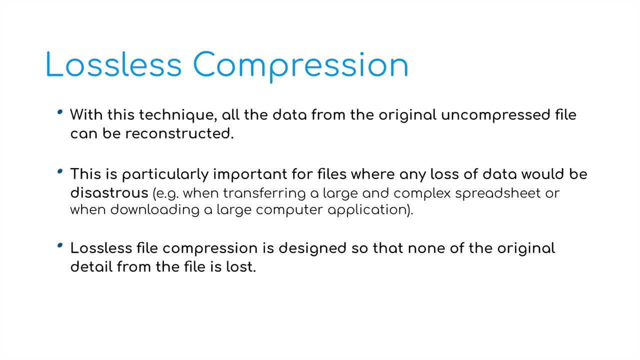 compress is the same as what you get back when you uncompress it. It's particularly important for files where any loss of data could be disastrous. I mentioned before Python programs, but things like complex spreadsheets, things like databases would all suffer if they were. 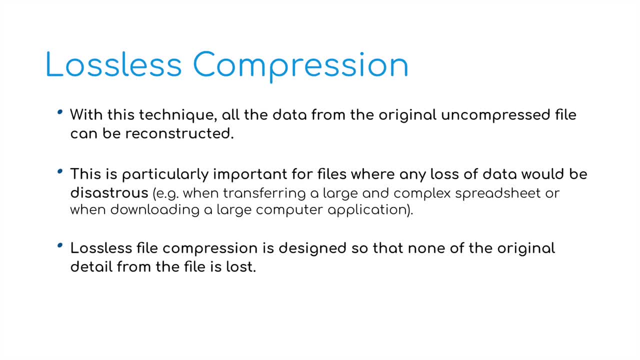 compressed using lossy compression. Lossless file compression is designed so that none of the original detail from the file is lost. But how does that work? Well, the first thing you need to do is to go to the main types of lossless reversible file compression, The one that's described in detail in the 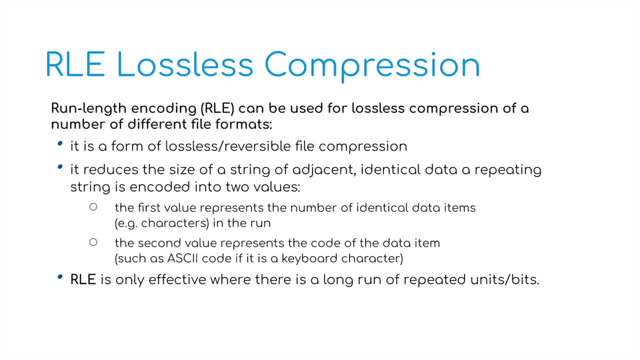 book is known as run length encoding or RLE. Now, this looks at strings of adjacent, identical data or identical characters and encodes them into two different values. The first value represents the number of identical data items and the second value represents the code of. 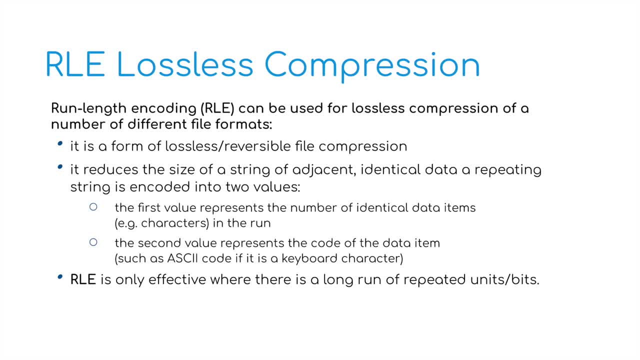 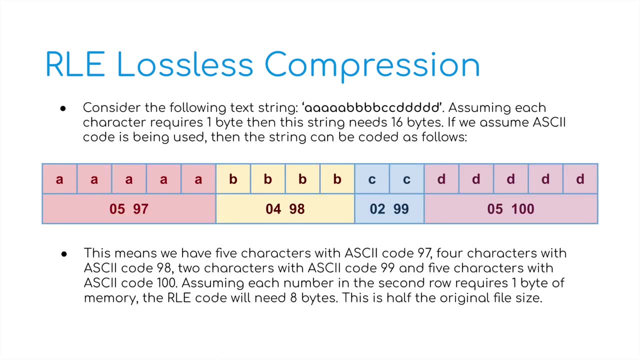 the data item Using ASCII code for particular keyboard characters. it's only effective where there is a long run of repeating units. So I'm going to show you an example. I've got some text. I mean, it's not really a word, It's just a group of A's, a group of B's, C's and D's, But 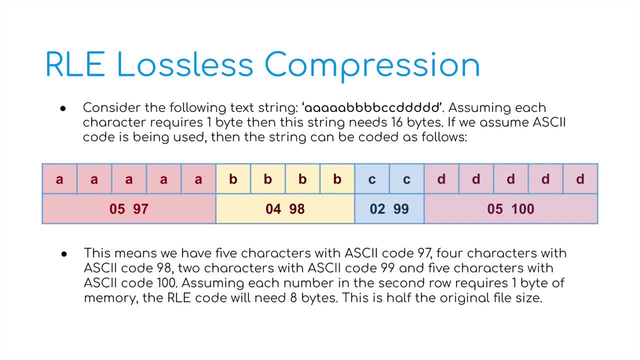 assuming each character requires one byte, then the string needs 16 bytes, the 16 characters. If we assume ASCII code is being used, then the string can be coded as follows: So we've got five lots of the value 97.. We've got four lots of the value 98.. You can see. 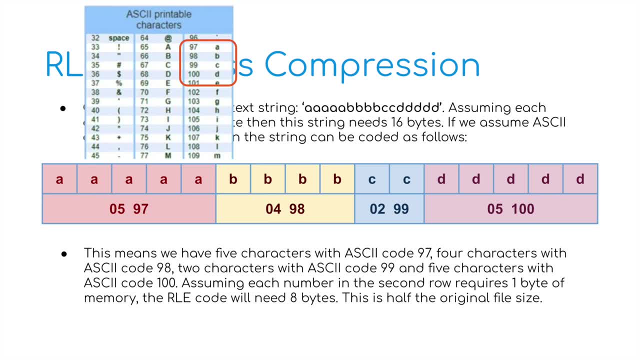 that on the little box. I've put on there the little reference: Two lots of 99, C and five lots of the value D100.. Assuming each number in the second row requires one byte of memory, the RLE code will need only eight bytes. So let's reduce it by half. We've 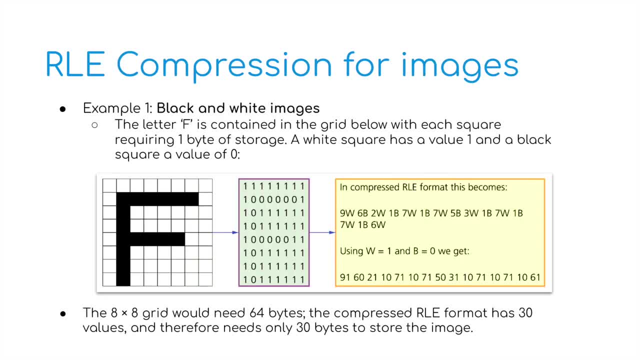 got 50% of the file size, Okay, Okay. Working Similarly for images, I've got the letter F. I've just got a black and white image here And, of course, this is one bit, Each one of these little pixels, each one of these squares. 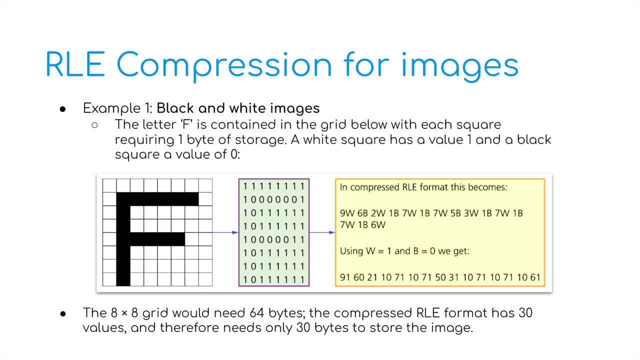 can be referred to as one bit of information. Therefore, it's either black or white, So I've separated this out into ones and zeros, As you can see there. So on the top row we've got eight lots of white of ones. if we use W to equal one. 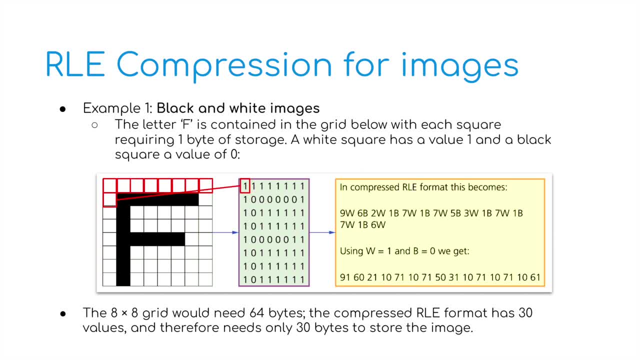 But we've got one. in the next row before the F starts, We've got another one just below it, So we've got nine ones, and then we've got the black section, which is obviously six blacks, and then two more whites, a black. We carry on, and carry on, and carry on until 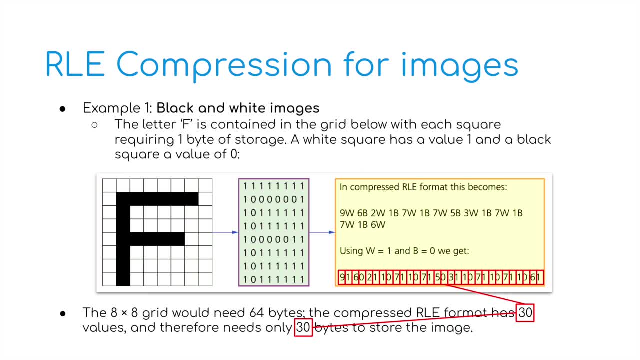 we getuntil, we can establish that the eight by eight grid dipped 64 bytes of information for that uncompressed file format. But if we work together here it makes more space. So we've added two neutrals and now, If we work in this manner, if we assign this number, then we can reduce it right down to only 30 bytes to store the same image. 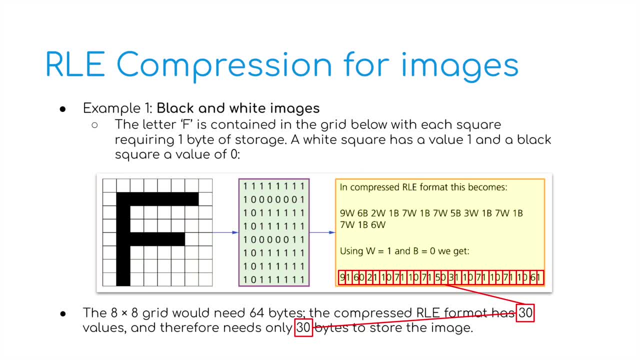 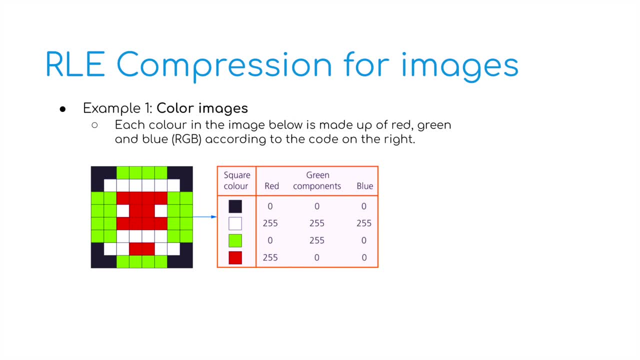 So again we've over half, over 50% compression there. If we look at colors- colored images- we can assign values again to this And I've got a complicated one again using examples from Cambridge. So we've assigned a value to each color. 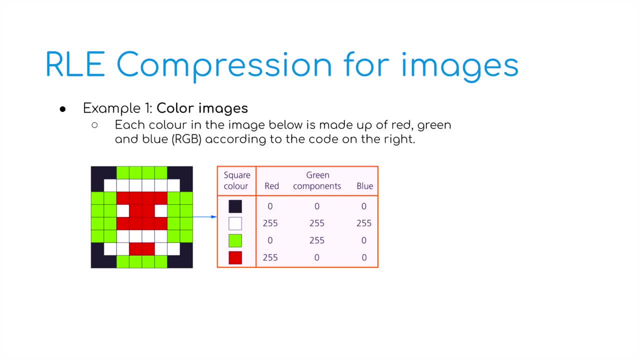 For example, black is 0, 0, 0.. White is 2, 5, 5,, 2, 5, 5,, 2, 5, 5.. The same as in RGB format. Green: no, lots of red. 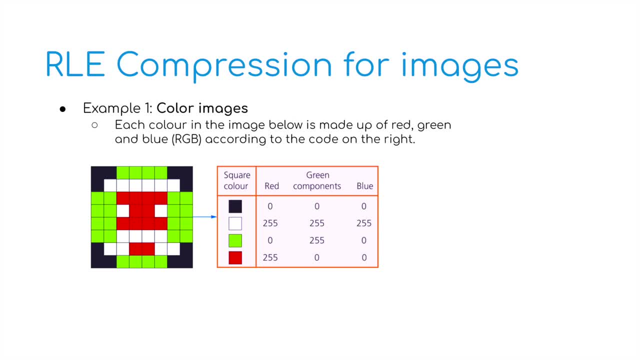 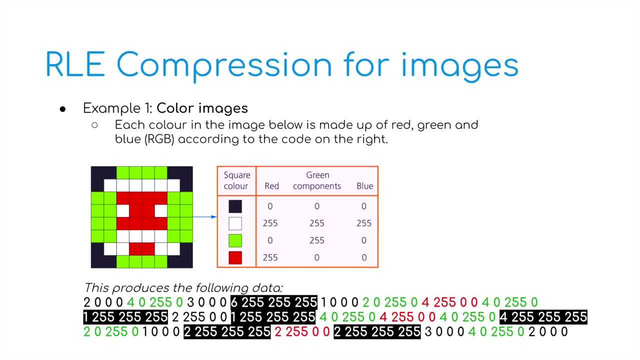 Full 2, 5, 5, green, No lots of blue. Red, 2, 5, 5, red, Zero green, zero blue. So what have we got here? Well, if I start with the top one, we've got two lots of black. 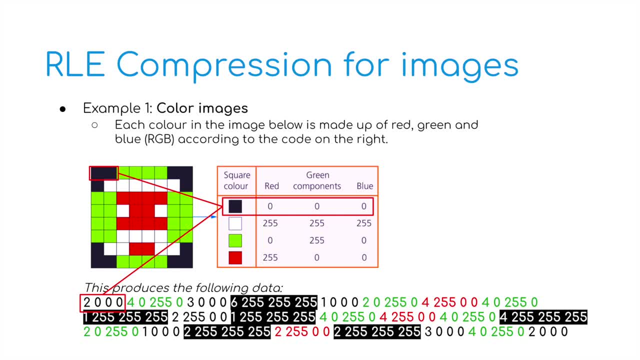 Two lots of 0, 0, 0. Then we move on to the next one, We move on to four lots of 0, 2,, 5,, 5, 0.. And then back to black again, And we continue, continue, continue. 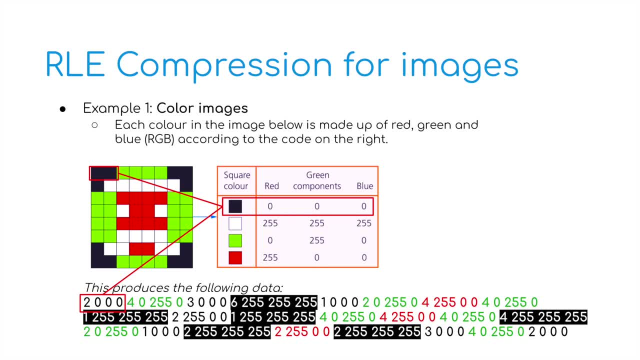 So the original image, 8 by 8 square, would need 3 bytes per square. This incorporates the RGB values. Therefore, the uncompressed file for this image would be 8 times 8, 64, times 3, 192.. 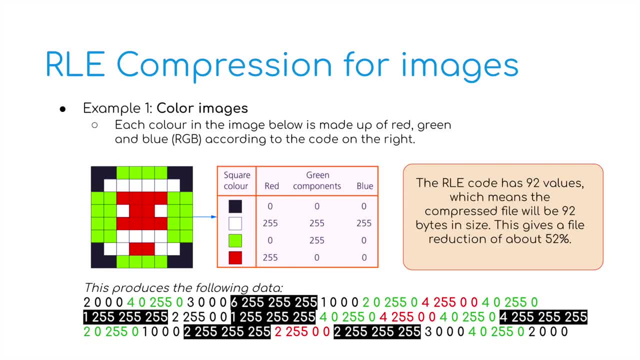 But the RLE code is only 92 values, which means that the compressed file would then become 92 bytes. So therefore, again, we're reducing it. We're doing quite well here. We're reducing it by about 52%. 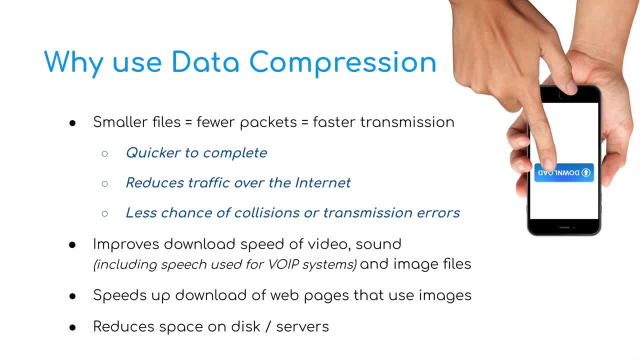 So that's fantastic. So just to recap, we've been through lossless, We've been through lossy compression. We know the differences. We know that one potentially loses data, loses quality, loses information, And the other one, lossless, retains everything that. 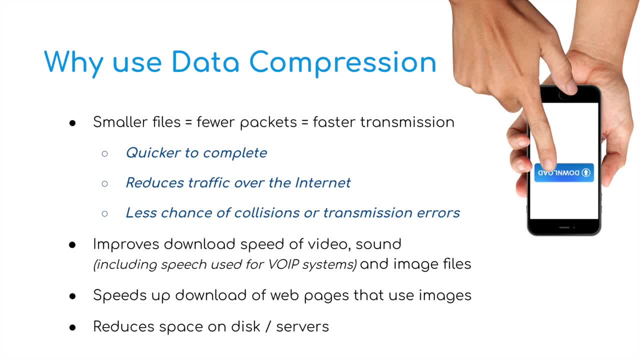 you know we started with. But why do we use data compression? Well, it creates smaller files, which equals smaller packets, which equals faster transmission. Therefore, it's quicker to complete. It reduces traffic over the internet. There's less chance of collision or transmission errors. 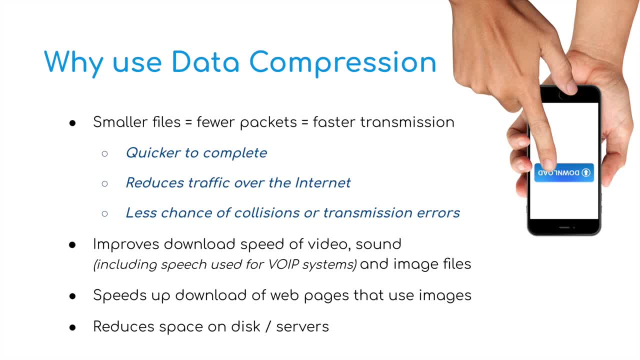 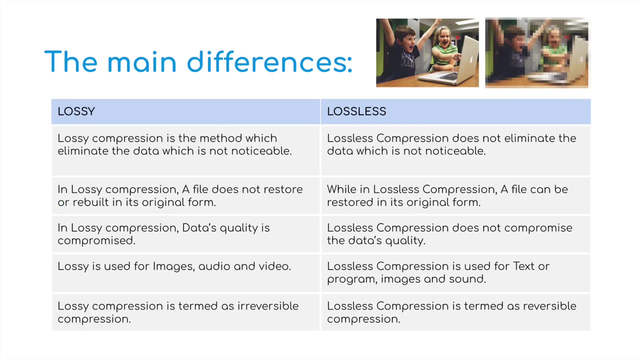 It improves download speeds of video and sound, including voice over, IP systems and image files. It speeds up downloads of webpages that uses lots of images And it reduces loss. It reduces the space on your hard disk or on the server. Now we've got here a little table just to finish off with. 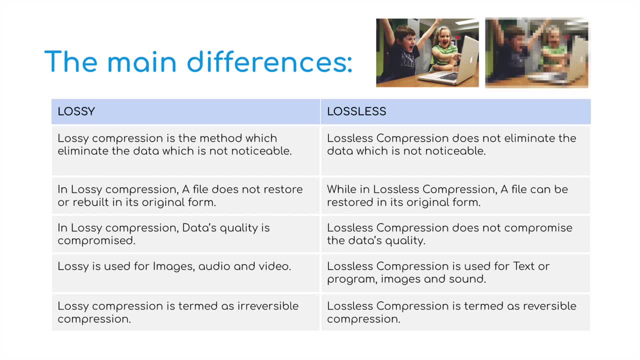 about the main differences And I'll just read this out to you. So lossy if we compare the two. lossy compression is a method which eliminates the data which is not noticeable. Lossless compression does not eliminate the data which is not noticeable. 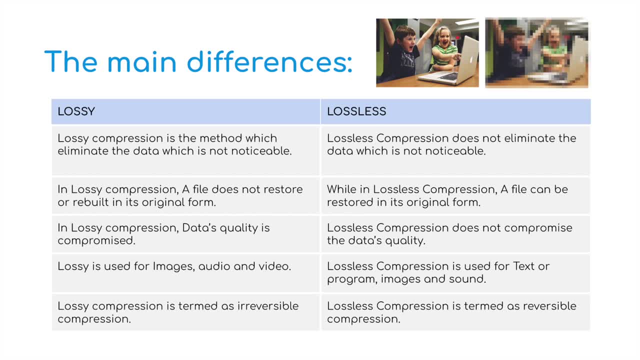 Okay, that's fair enough. In lossy compression, if you were to do a comparison on an exam paper, in lossy compression a file does not restore or rebuild to its original form, whereas in lossless it would do. In lossy compression, data quality is compromised.